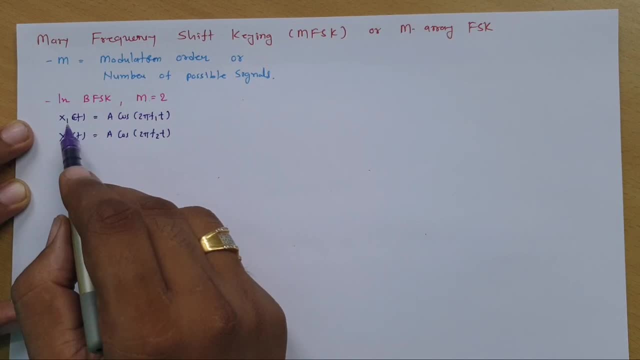 F2t- those are two different carrier signals- which is representing X1 and X2, right, And if I down that two Og and like right and which one, it is the current common assuming question, right. So it is there two common common questions, right. And then if I say A cos of 2 Pi, F1t, have two signals. one signal is X1 and second signal is X1, t right, and its sisging 2 Pi's, so right. So if I have to claim, recognize right, Then the boundary is given by the denominator of S. Now if I have to, 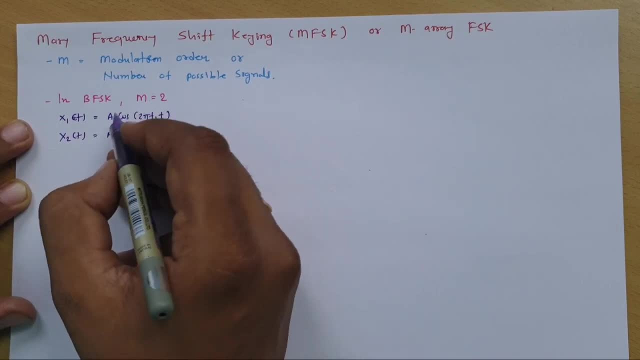 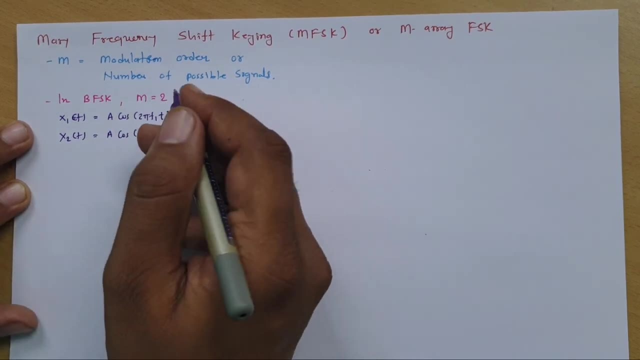 second must be defined between Wars favor, then A cos 1t, that is, A cos 2 pi from 1 to F2 t, then the other. and if you see my session based on bpsk, where i have derived amplitude in terms of energy per bit, and if i want to write that in that form, in that case that will be square root of 2 e b. 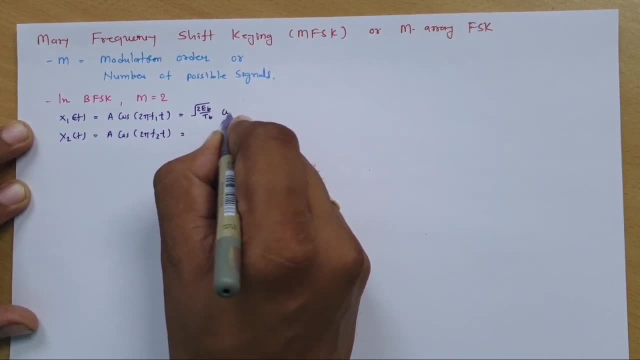 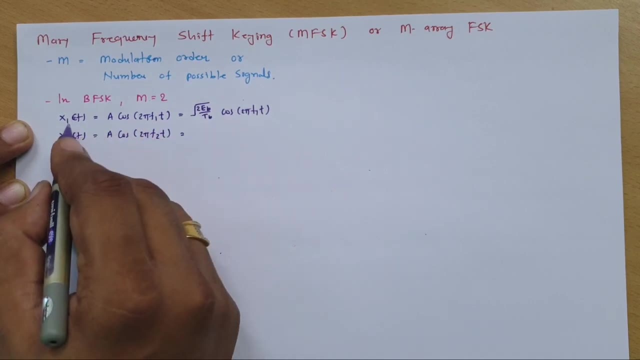 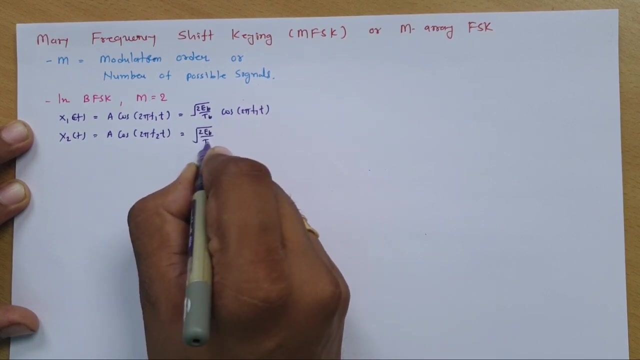 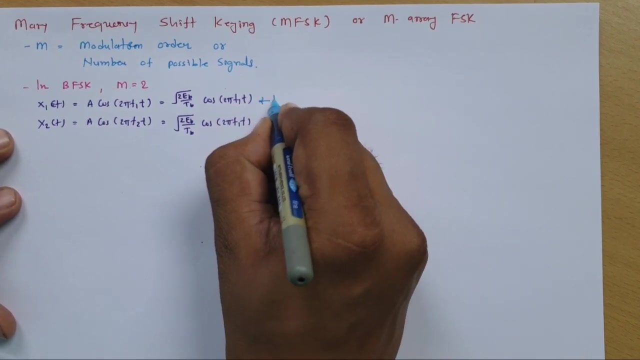 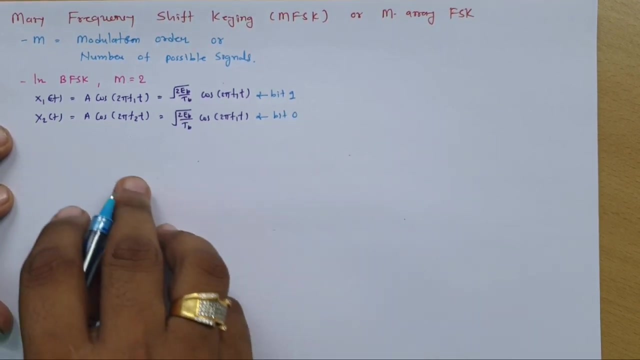 divided by tb into cos of 2 pi, f1, t right, where f1 is frequency associated with x1 and f2 that is frequency associated with x2 right and in bps b, fsk. here this x1 is representing bit1, so this is representing bit 1 and this is representing bit 0. so that is what the case. 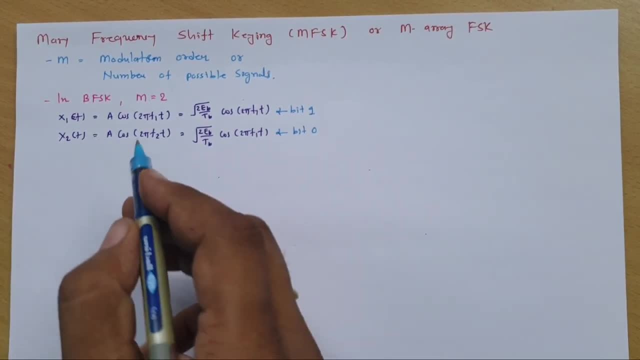 which is there in terms of equation. now, if you increase modulation order, then you will be finding number of carriers will increase. right, and usually modulation order will justify number of bits per symbol. even so, if i say i have m different signals, then from that we can identify how many. 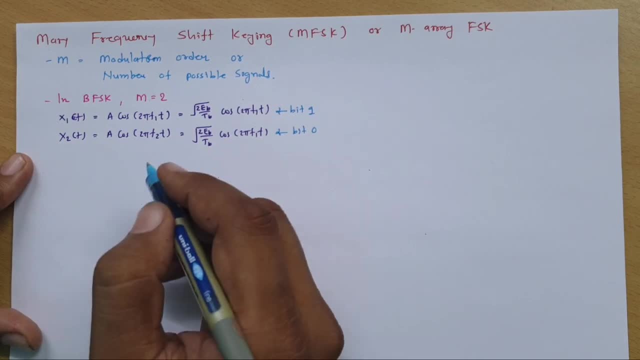 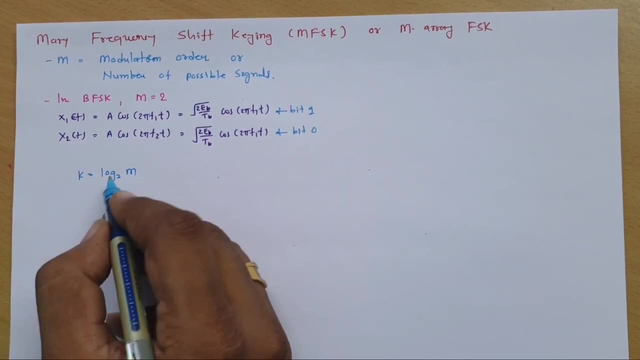 number of bits are required to represent given symbol, and for that, basic formula is: k is equals to, k is equals to log m base 2. right, and here we can say this: k is number of bits per symbol. right, and here we can say this: k is number of bits per symbol. 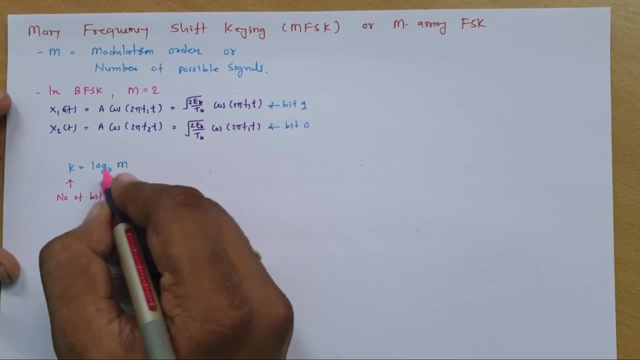 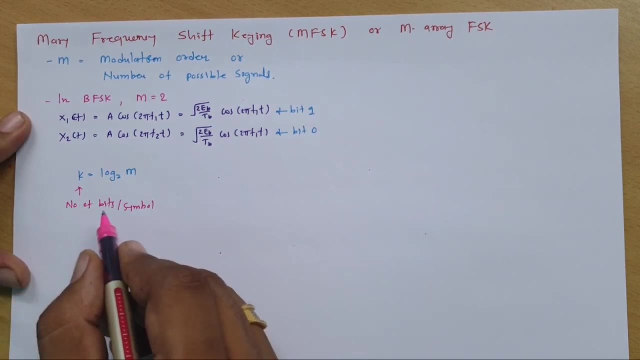 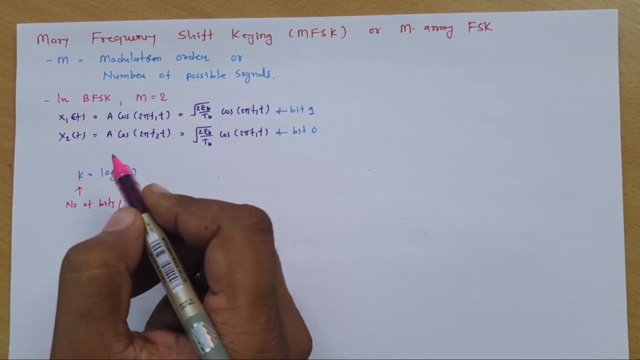 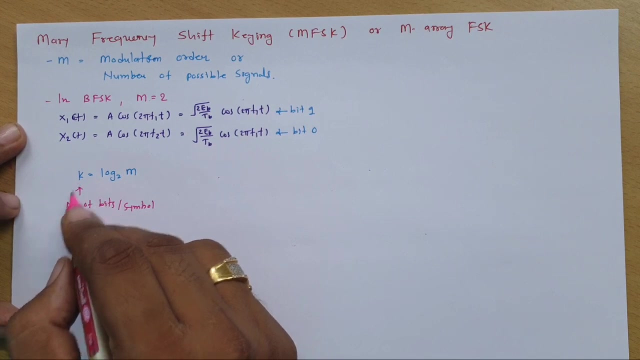 and m is modulation order right. so that is how we can identify how many bits are required to represent given symbol, and that is what a signal that one can say right. so here see, for example, if i consider k is equals to 2, in that case we will be having: m is equals to 4. or one can say: if m is 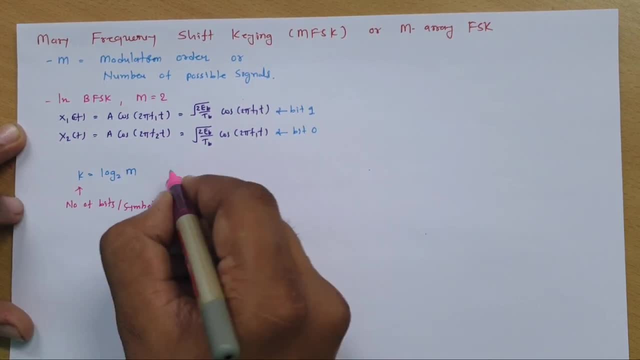 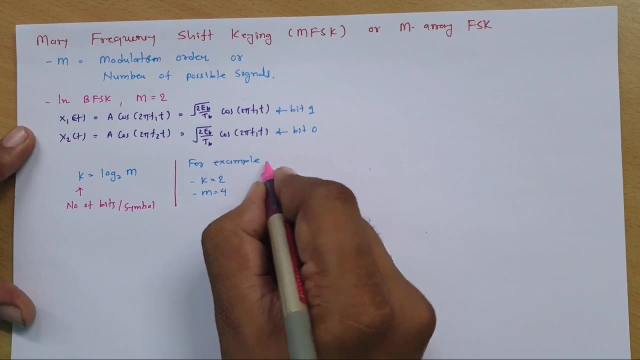 equals to 2, then we will be having m is equals to 4. or one can say: if m is equals to 2, then we will be having m is equals to 4. in that case k is equals to 2, right? if you want one more example, then for m is equals to 8. 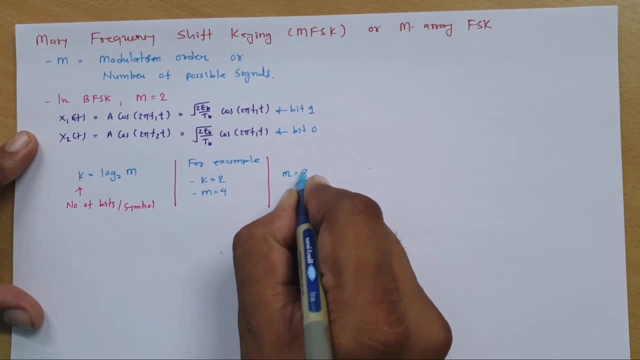 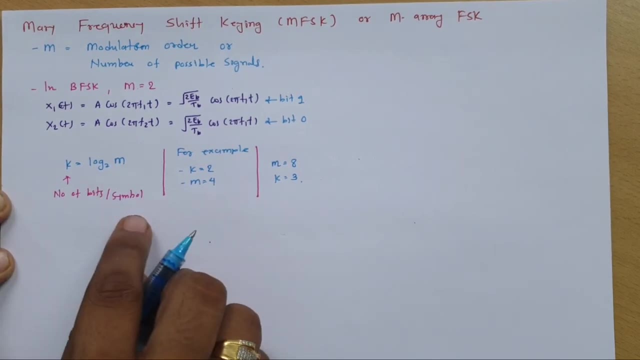 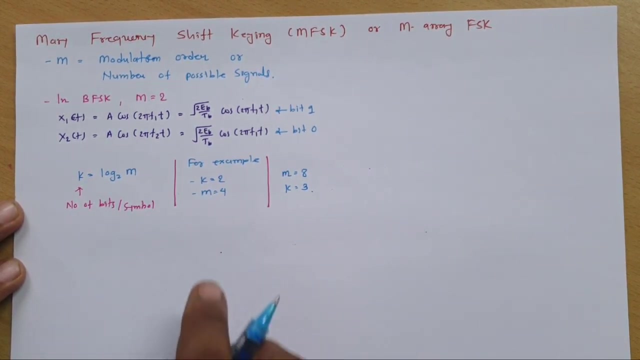 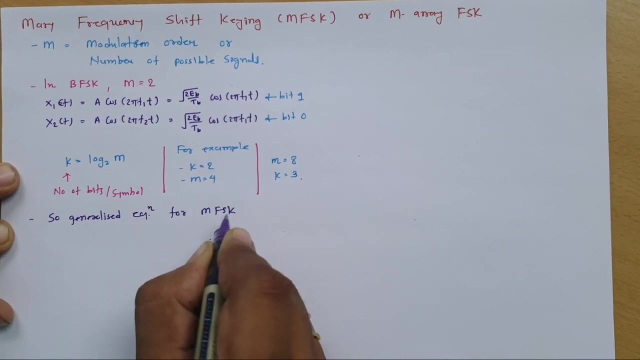 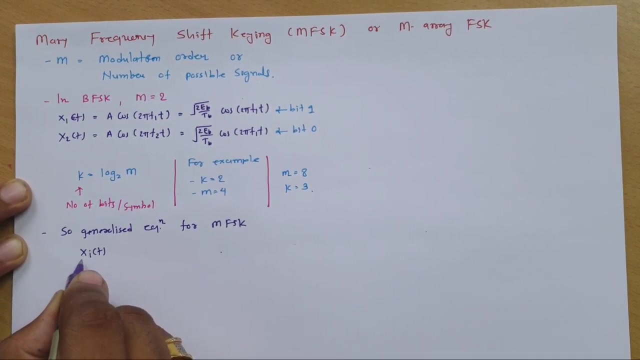 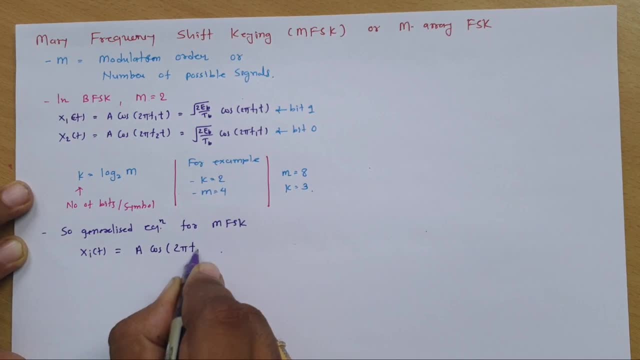 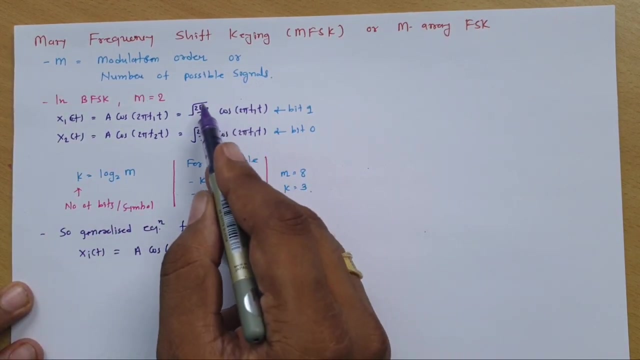 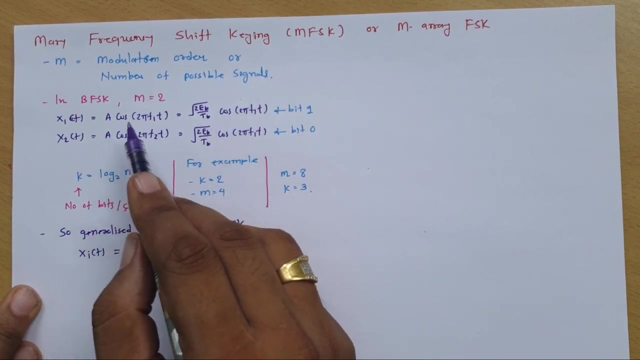 a cos of 2 pi fit right where. now you see this time period, that will be associated with symbol. it is not associated with bit see for binary. one can have this time period associated with bit duration, right? so for this case there are two symbols only. so here this time period. 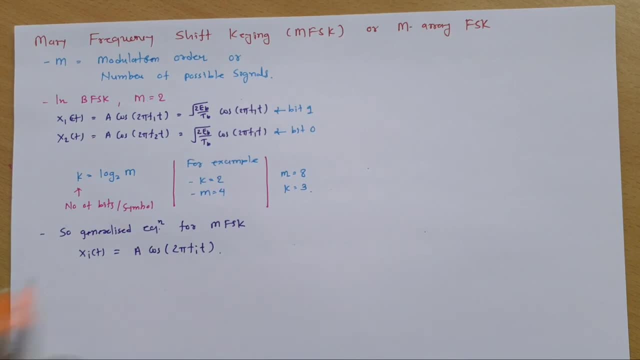 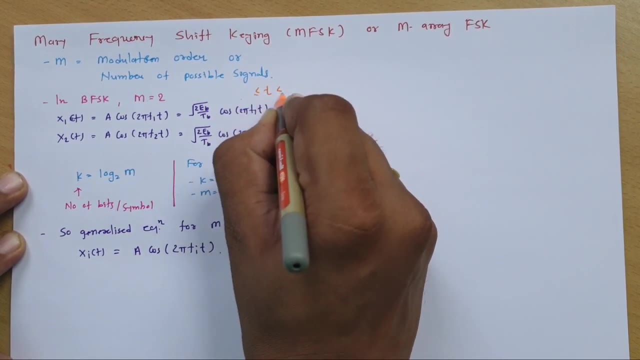 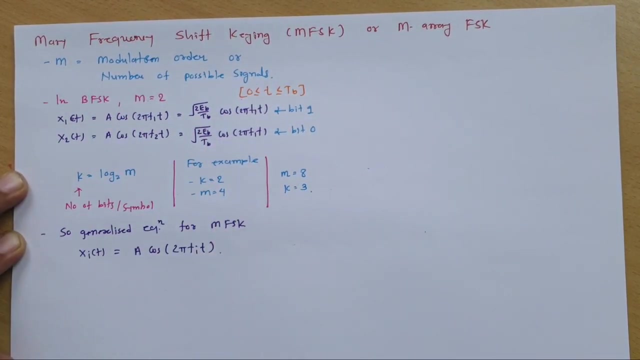 that is there in the vicinity of 0 to tb bit time period. right, where here this t that was there in between 0 to tb, as it was the case of bpf, b, fsk, but when we talk about mfsk, in that case this time period that is associated with symbol duration, right. 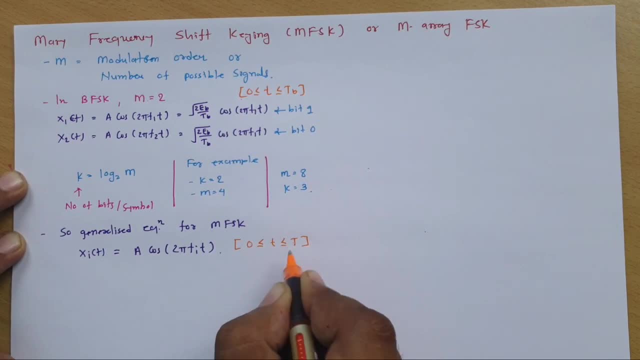 where this t, that is symbol duration, and this tb, that is bit duration. so this is one difference that one should know. and i is what ith symbols frequency? i is ith symbols frequency, right, and here how to identify ith symbols frequency. so for that, to identify ith symbol frequency. 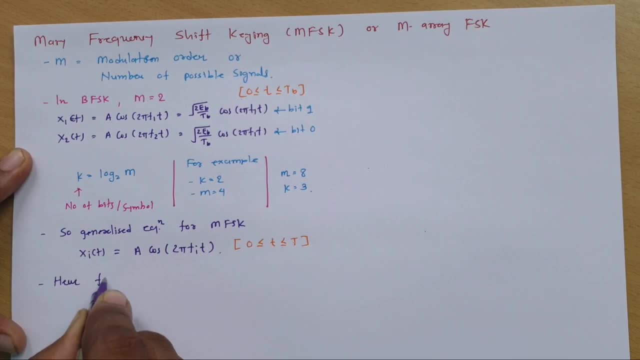 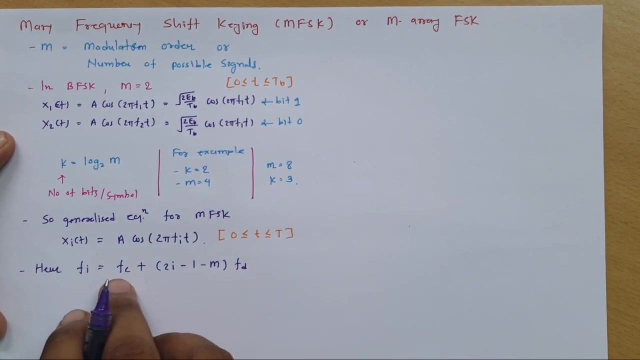 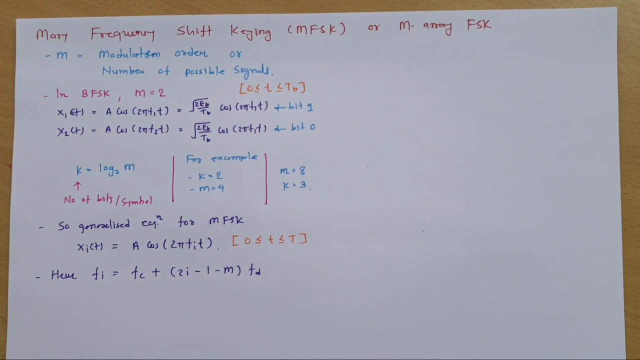 here fi is equals to fc plus 2i minus 1, minus m, into fd, where here fd is frequency deviation, fc is center frequency, fi is ith symbols, frequency right, m is modulation order. so that is how it is there. so let me mention all those data so it will be more clear. so fd: 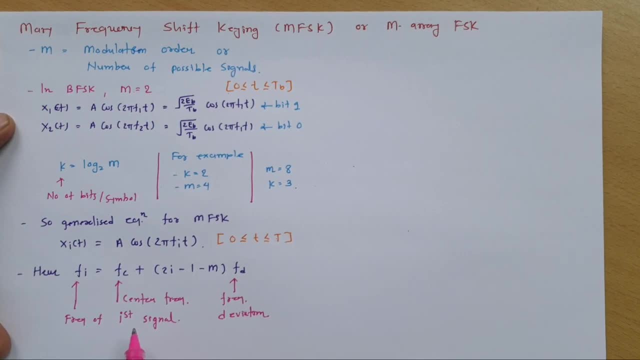 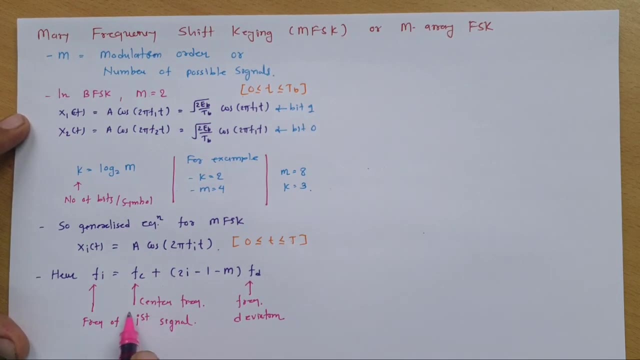 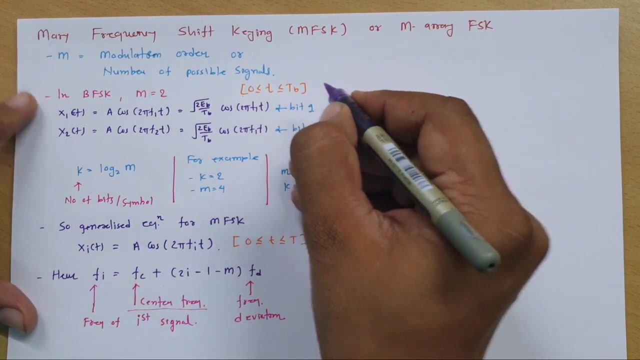 is frequency deviation, fc is center frequency of ith center frequency and fi is frequency of ith signal. right, so that is how this fi can be determined. now let us have one example, and based on that example, i will explain you how we can utilize this mfsk. so see, there is one example that is given to us, so let 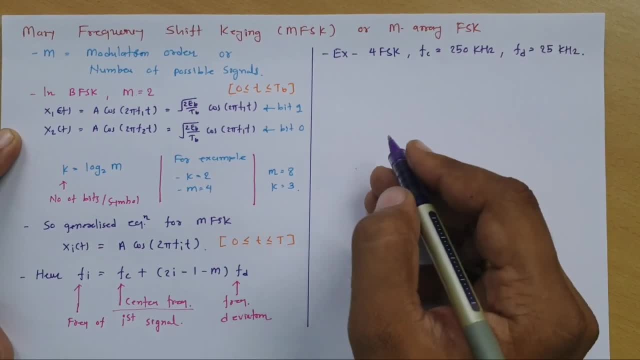 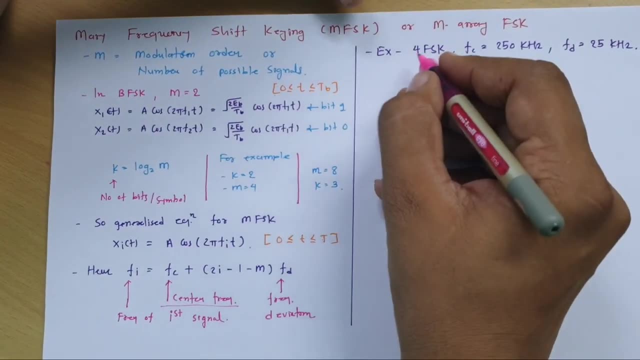 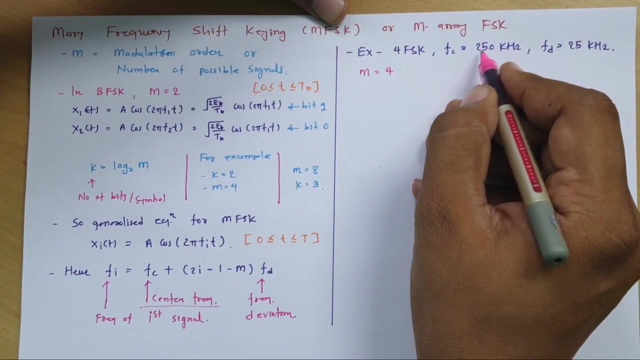 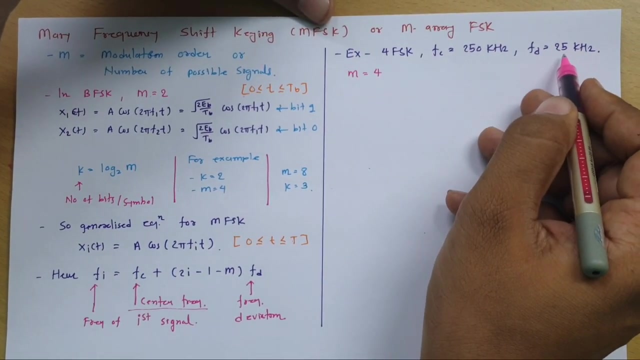 me write question over it. so here 4 fsk is given right. so based on that we can say: 4 fsk means m is equals to 4 and center frequency that is given. so 250 kilohertz center frequency and fd means frequency deviation, that is 25 kilohertz. that is given to us and 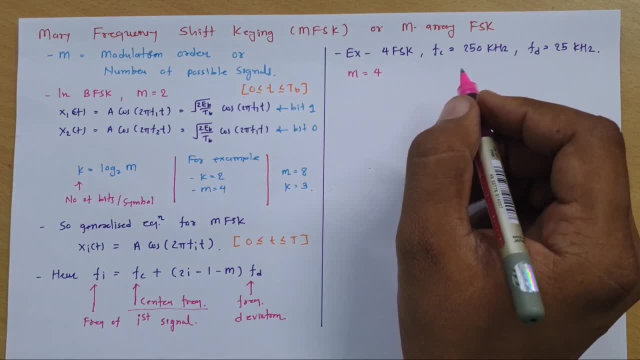 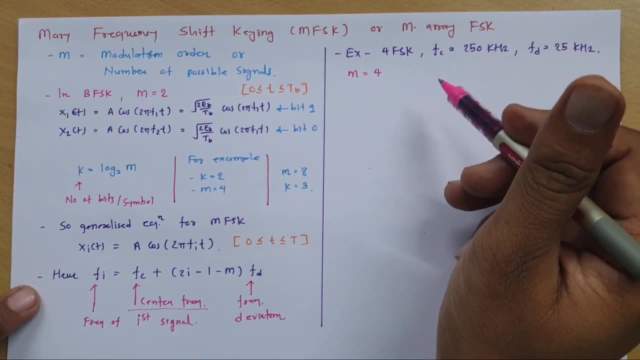 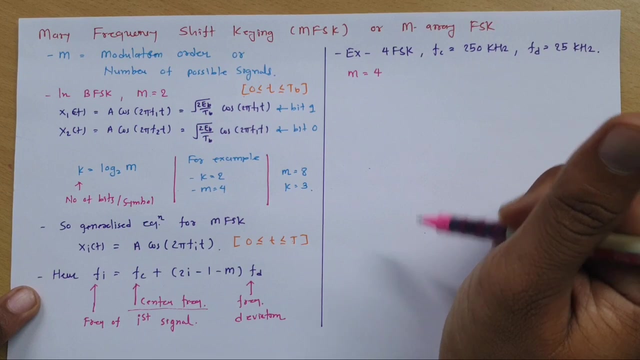 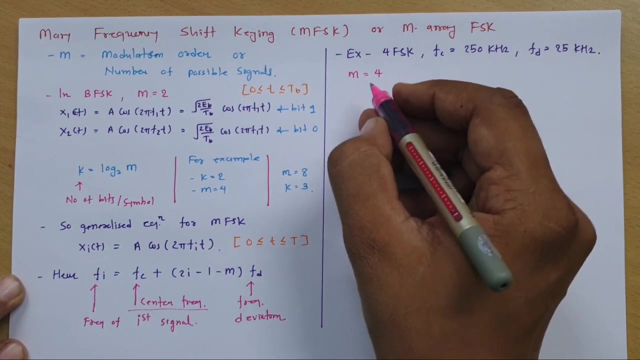 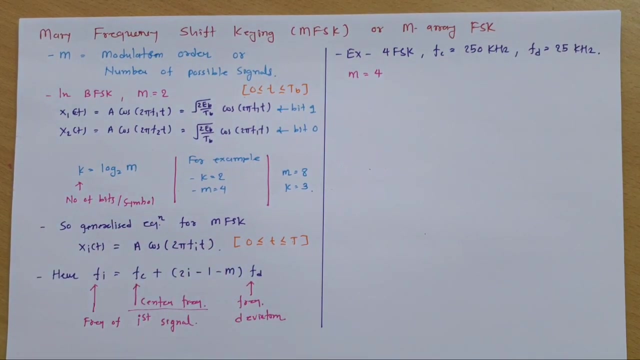 our agenda is to identify how many frequencies are there with different symbols. secondly, how we represents number of bits per symbol and what are the bits. that is what we are giving it to, given frequencies. So see here, as per this basic formula, k is equal to log of m. base 2, we can identify number. 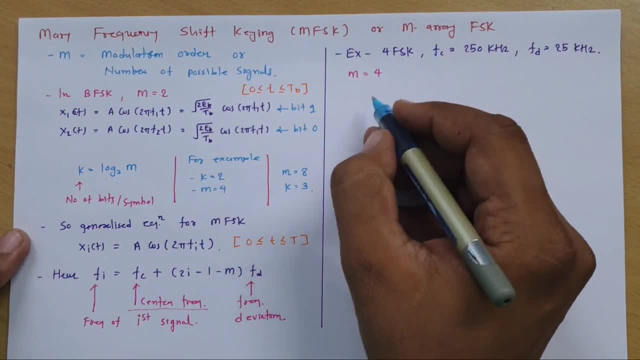 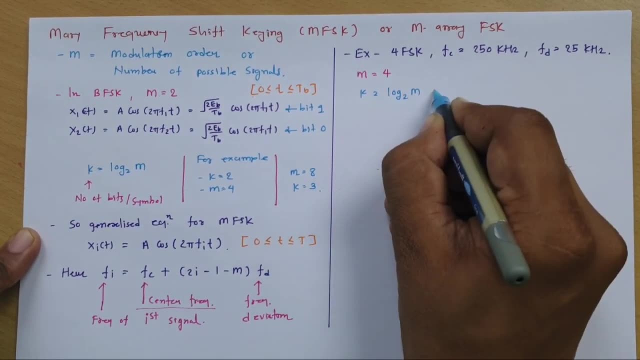 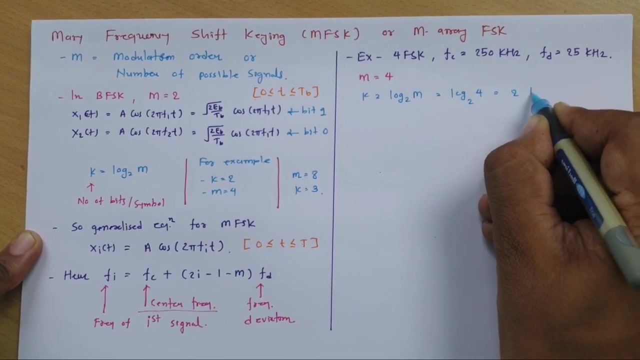 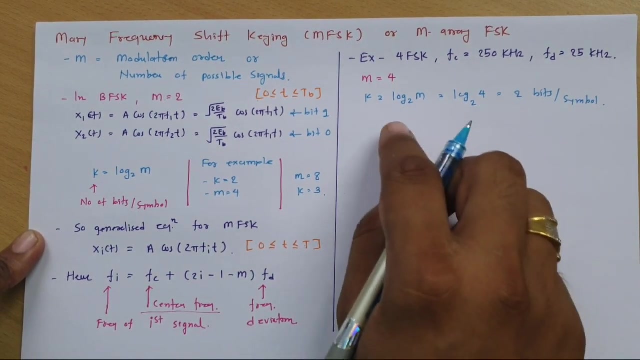 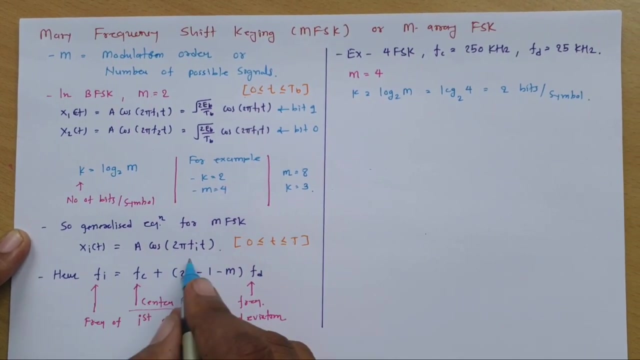 of bits required per single symbol. so k is equals to log of m base 2.. So if you place log of base 2. to four, so this is what two means two bits per symbol that we need to have right now. as this is four fsk, there are total, four frequency, which is there as per this equation, where fi that will be. 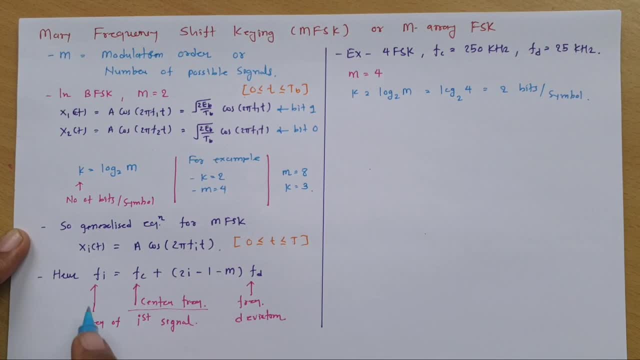 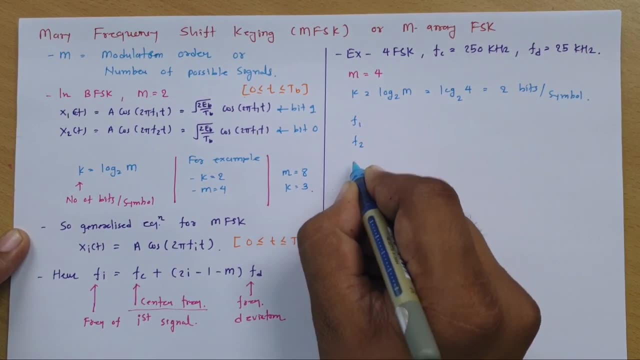 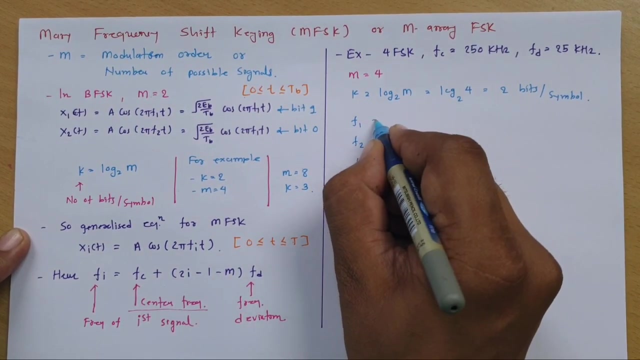 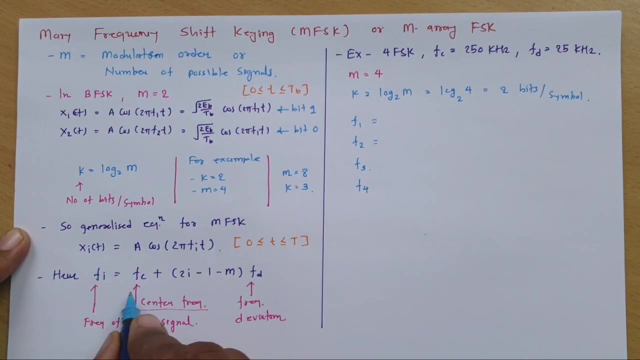 f1, f2, f3, f4. so let us identify all those four frequencies, right? so f1, f2, f3 and f4, that is what the case which we are delivered to calculate and see basic formula that is: fi is equals to fc plus 2i, minus 1, minus m, into: 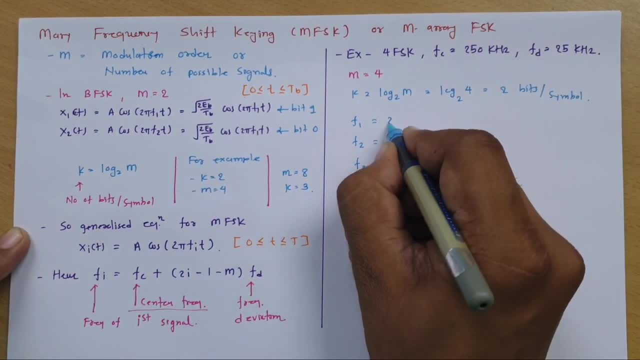 f1, f2, f3, f4. so let us identify all those four frequencies, right? so f1, f2, f3 and f4. that is what fd, right so fc, that is fix. that is 250. at the end i'll write: that is there in terms of kilohertz. 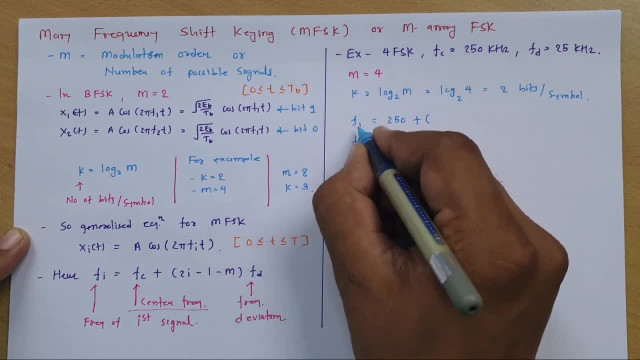 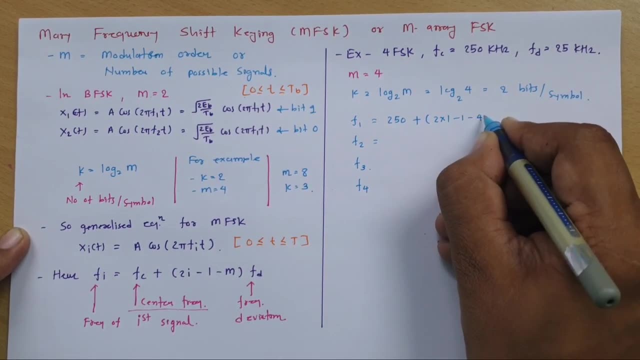 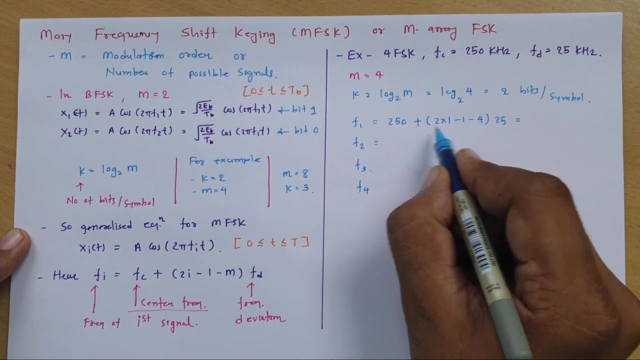 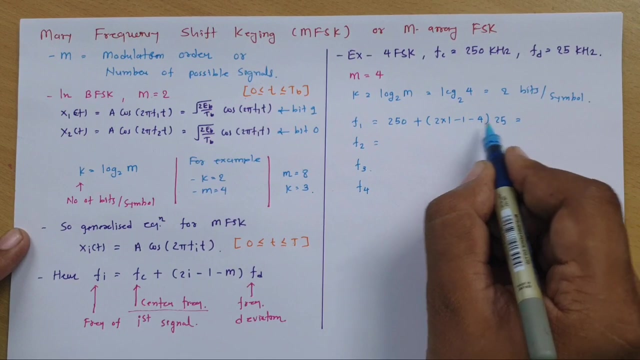 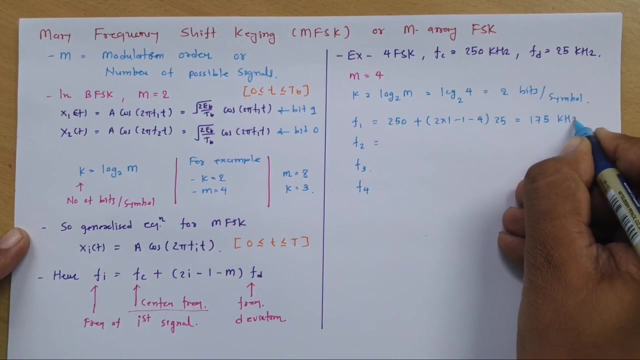 plus for first, it will be 2 into 1 minus 1, m is 4. so minus 4 into fd, that is 25. so see, this is what 250 plus 2 minus 1 minus 4 means. it is minus 3 into 25, so minus 75. so 250 minus 75, that is 175 kilohertz. now for f2, we can. 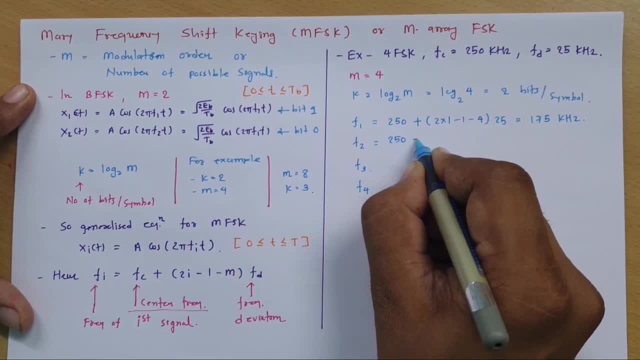 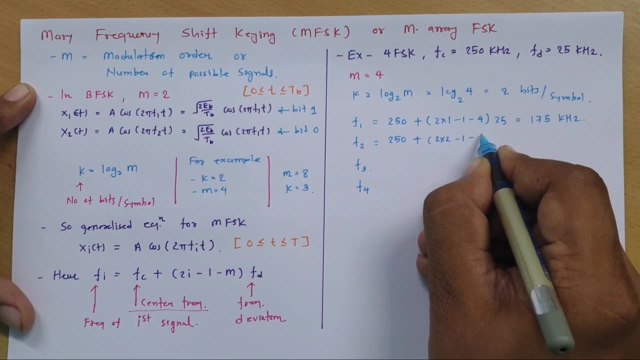 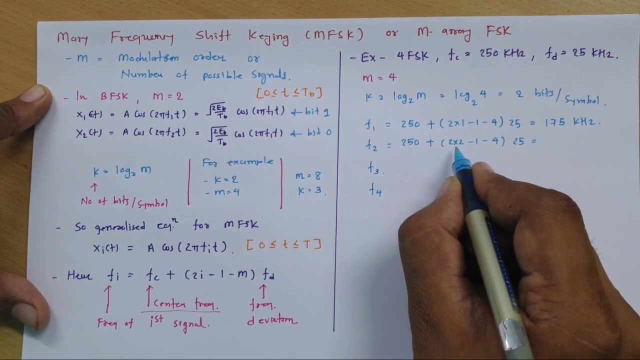 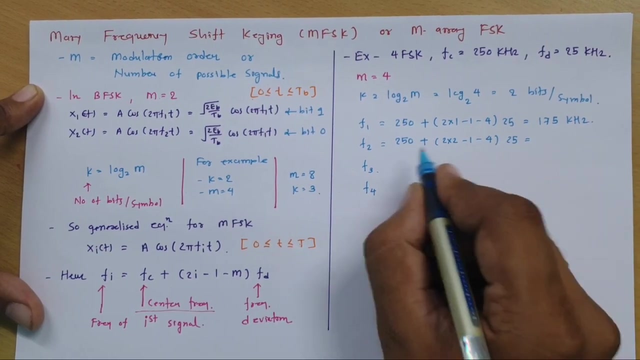 say it is 250 plus 2i, so i is 2 over here. so 2 into 2 minus 1 minus 4 into 25. so this is 250 plus 4 minus 1 minus 4, so that is minus 1 minus 1 into 25, that is minus 25. so 250 minus 25, that is 225. 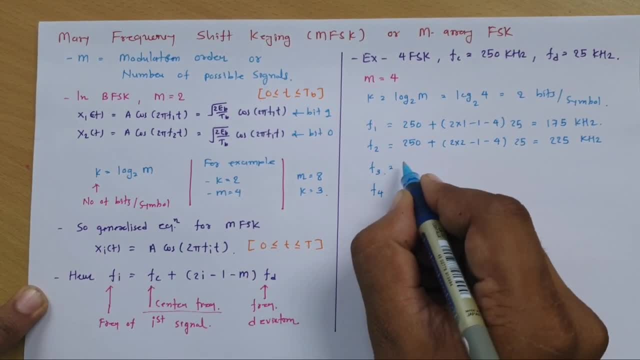 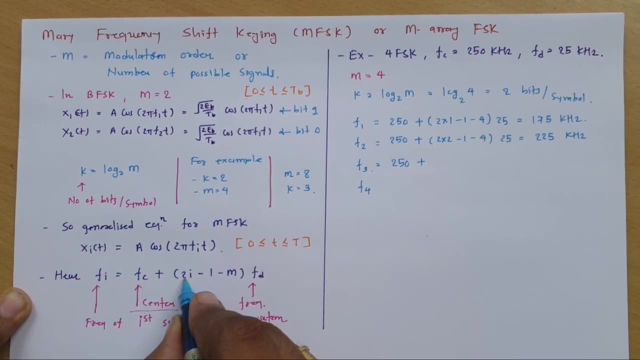 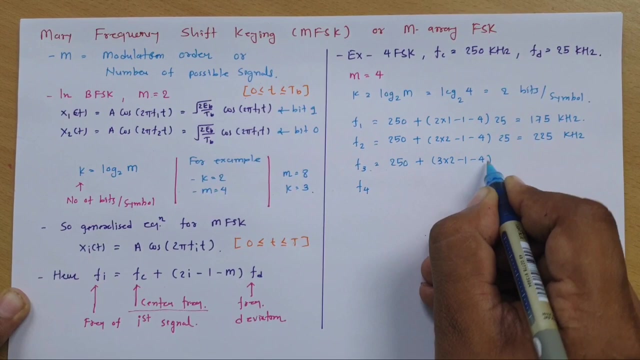 kilohertz, now similarly f3, that is 250 plus 3 into 2 right, so 3 into 2 minus 1 minus 4 into 25, so 6 minus 1 minus 4. so that is 1 right, 1 into 25, that is 25. so 250 plus 25, that is. 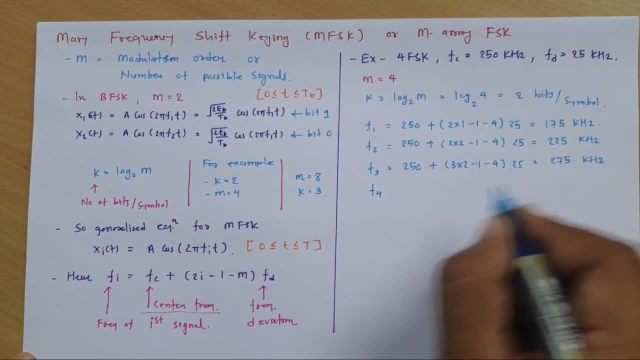 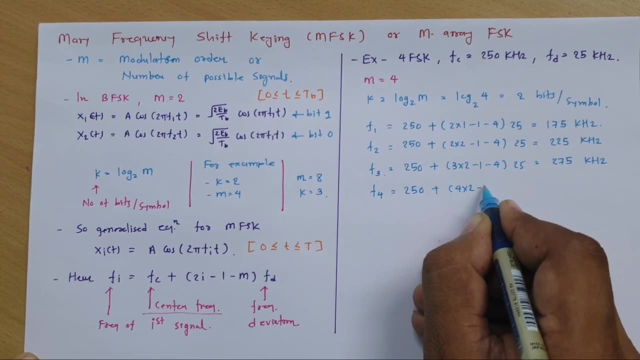 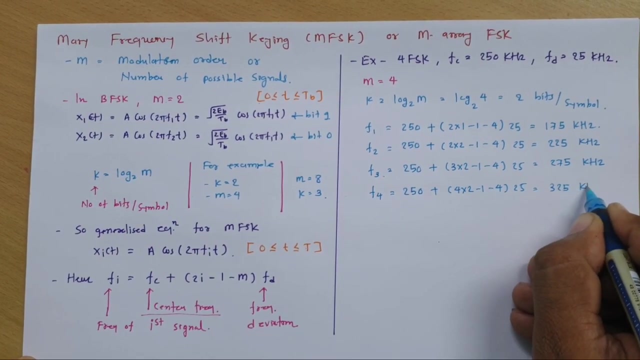 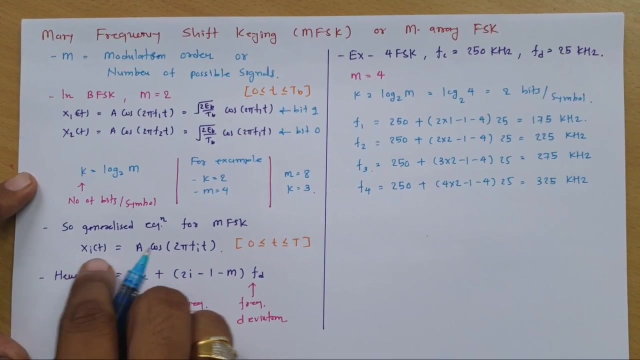 275 kilohertz. and similarly, fourth frequency, that is, 4 into 2 minus 1 minus 4 into 25, so that will be 325 kilohertz. so that is how, four frequencies that we can identify for this generalized equation. now, as i have told you, each symbol. 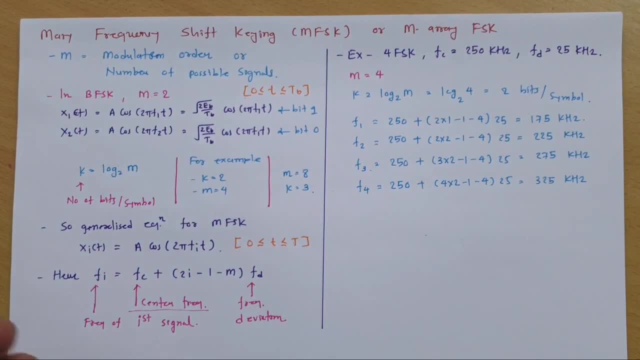 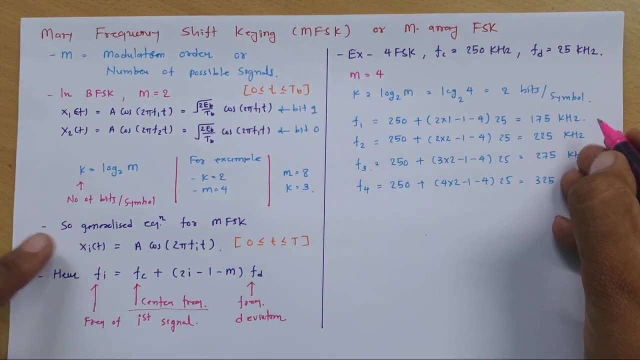 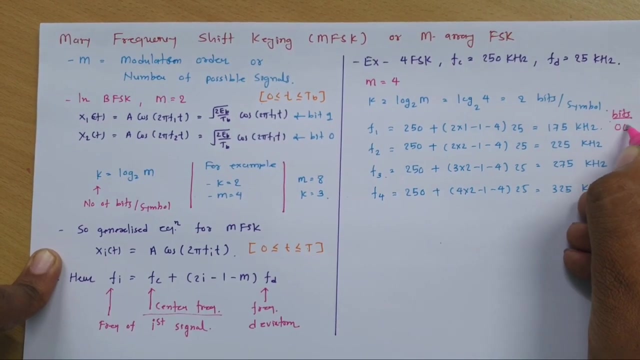 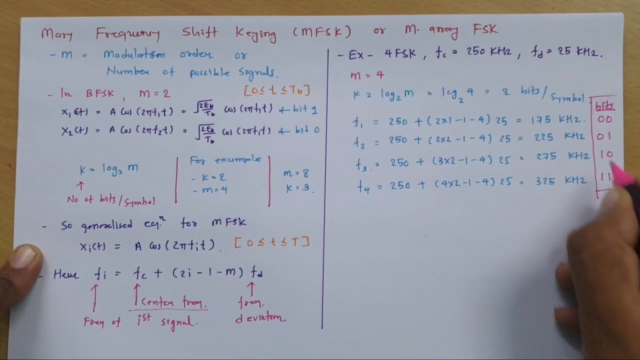 symbol will represent two bits, right? so here we can say: see, this is what first frequency that could have bits, two bits per one frequency, and that could be 0, 0, here it could be 0, 1, 1, 0, 1, 1. see, that is how we can send two bit at a same time for different frequencies. 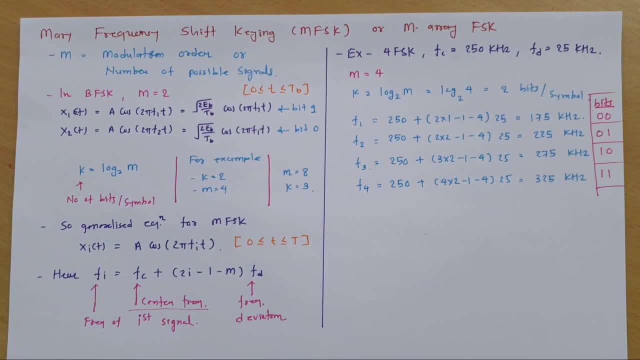 right, right now. see here, there are a few things which we need to take care of here. see, as there are four frequencies, center frequencies are there, four center frequencies are there, so at transmitter as well as at receiver side, we need to have four local oscillator. so let me mention it. 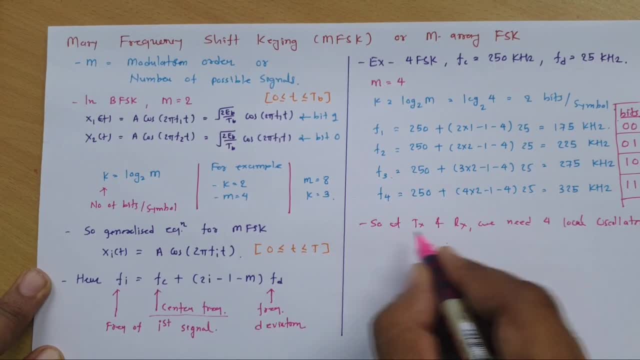 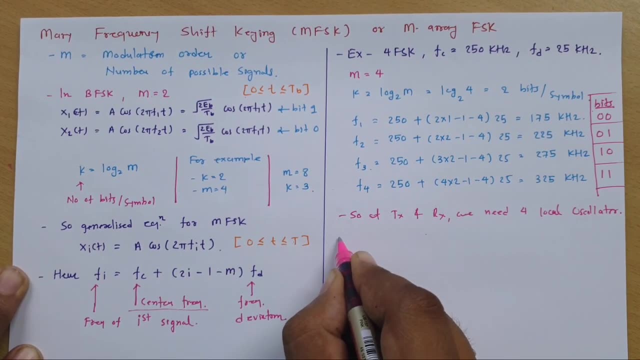 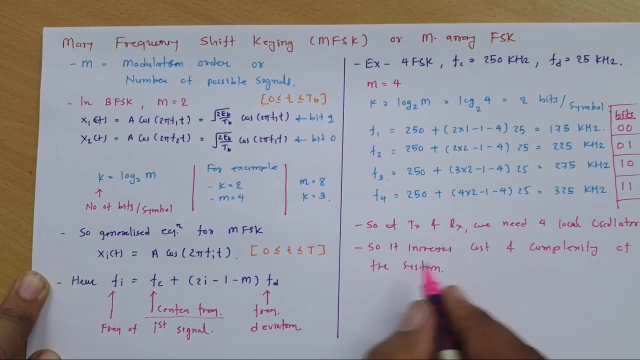 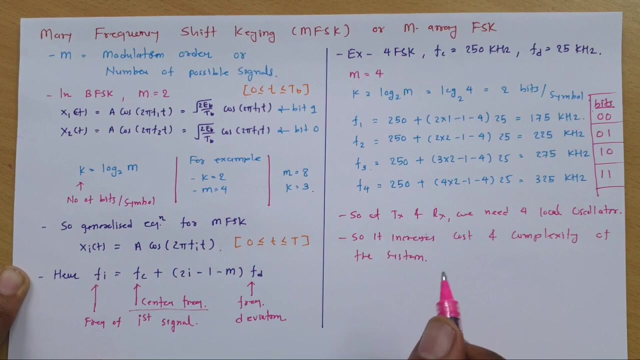 right and because of four local oscillators are required. it will increase complexity of the system and it will increase cost of the system. but you will be finding it is widely used in frequency whooping spread spectrum. so see, this is what we are using it in FHSS. it is widely used in 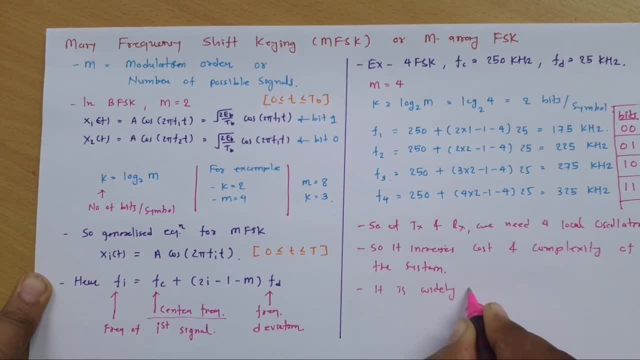 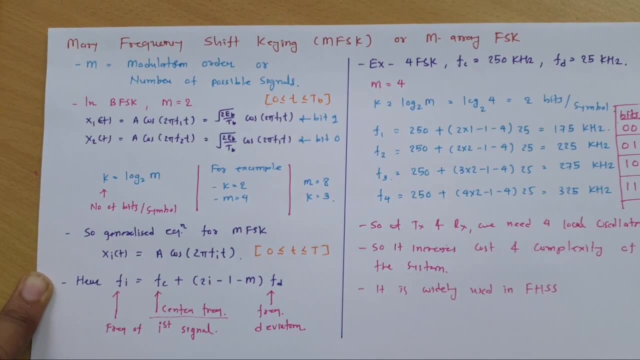 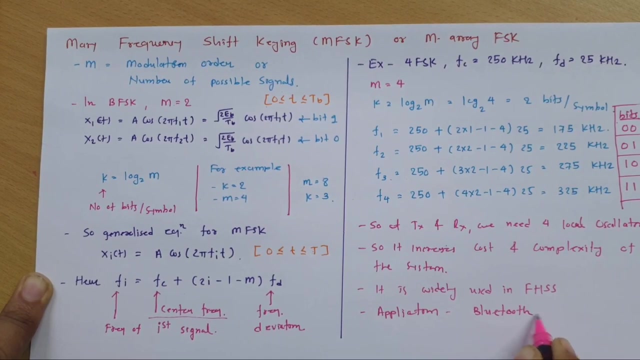 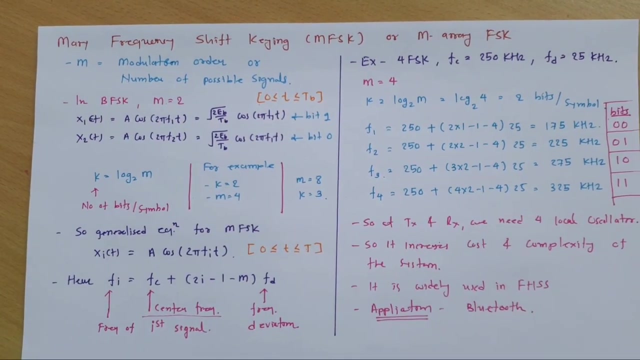 frequency whooping, spread spectrum and one major application, which is Bluetooth, that we all are using in our mobile phone, right? so major application that is Bluetooth. so this is what the case which is there with MFSK Mary frequency shift. King and I have made this session based on the request of students.